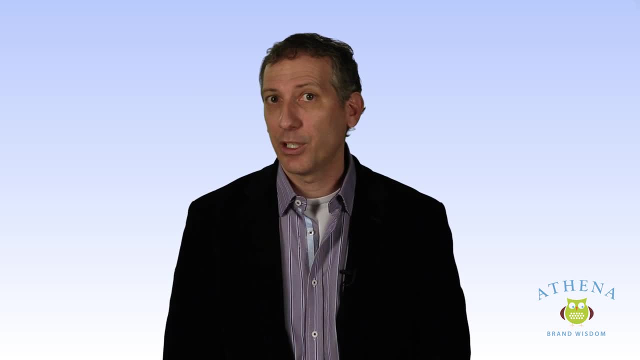 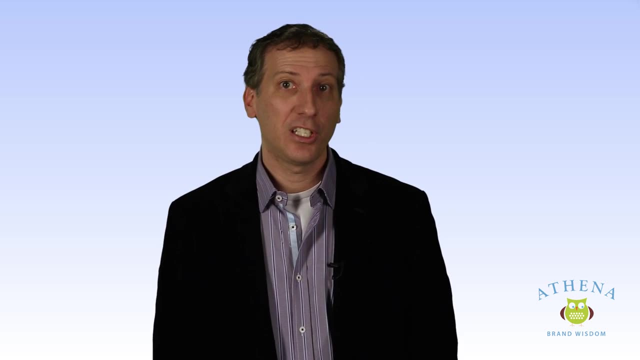 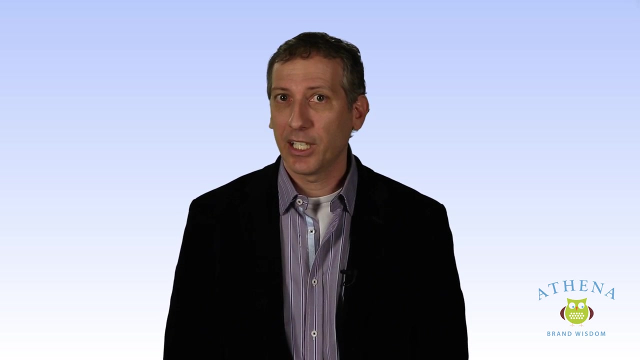 may probe with additional questions and works to make sure that they're verbalizing about the tasks they're doing rather than their opinions about the site. The reason this methodology is so effective is that it brings things that are otherwise hidden, like the internal planning, reacting and interpreting that people are doing while 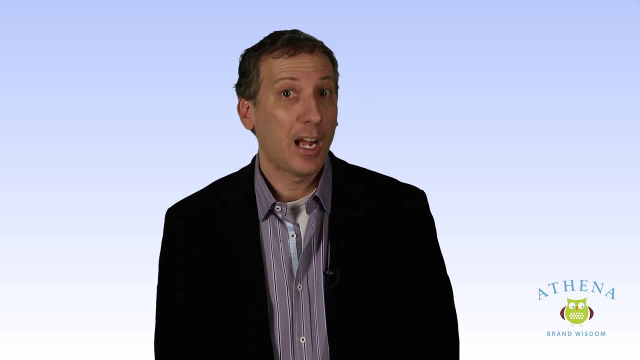 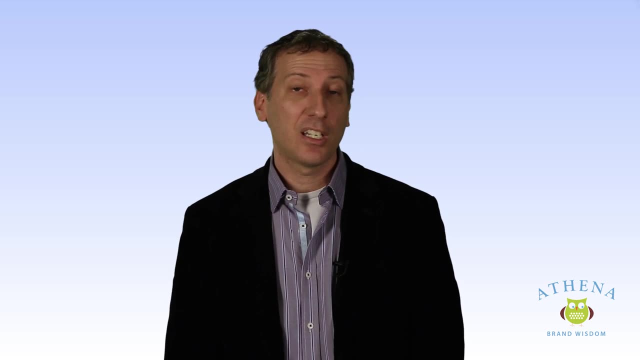 experiencing a site, things that are happening in people's minds out into the open where they can be observed and analyzed. So it's really just a dump of active memory. What we always observe when there is a usability problem is a disconnect between what people 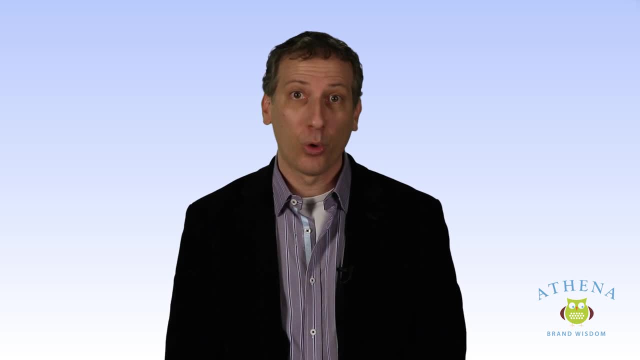 are thinking and how the site is interacting with them. and that's gold. A couple of other great things about the Thinking Aloud methodology. First, it's really impactful for designers to come face-to-face with consumers. Typically, we conduct this research at a market. 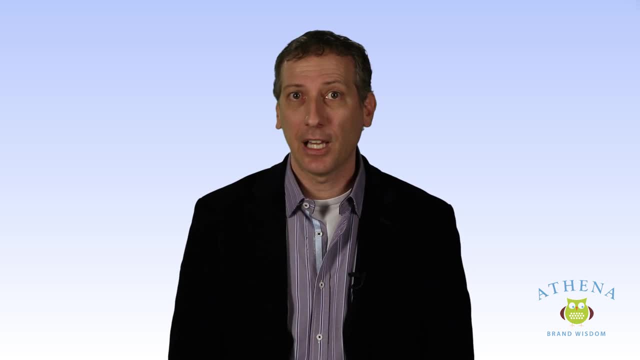 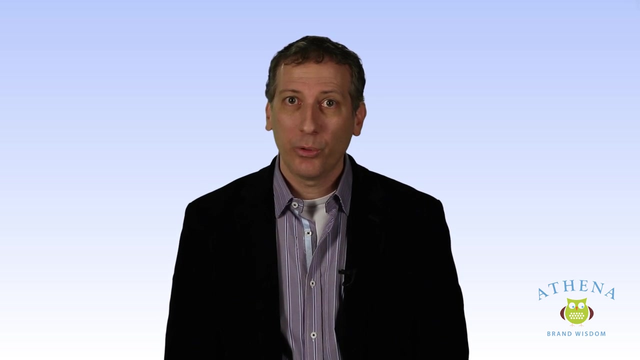 research facility with a one-way mirror where the designers are behind the glass, and we find the psychological impact of actually seeing a user. Seeing a user tripping over things on a site settles debates and leads to fast decision-making. Second, this kind of research is relatively fast and that's because you can do a solid. 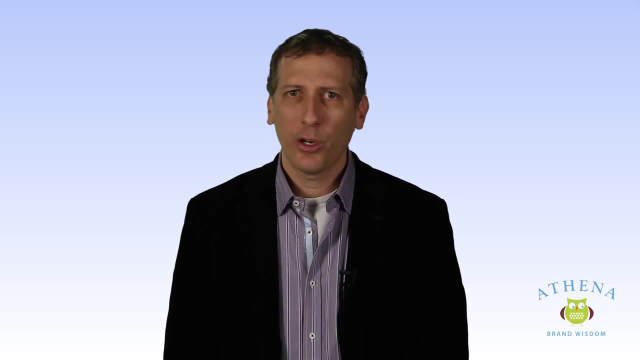 job of usability testing with as few as five users. I know that sounds lower than other kinds of research, and it is with good reason. If you're doing focus group research on people's opinions, you have to do a lot of people. 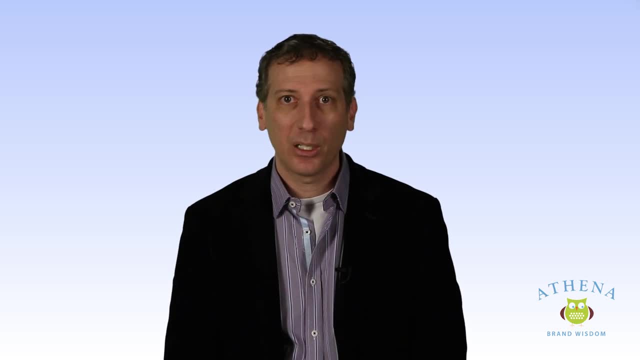 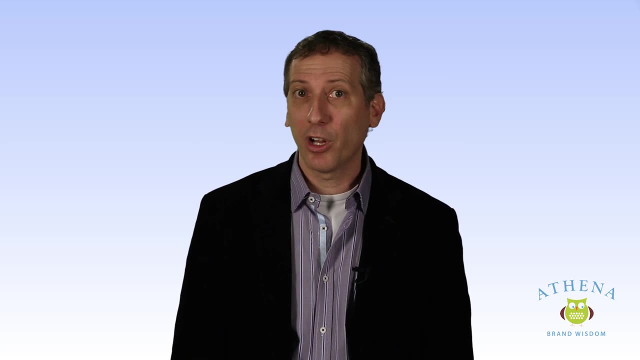 because opinions vary widely. but with usability testing, we're not uncovering opinions, We're uncovering behavior. We're not uncovering behavior. We're uncovering the way that we think. and the way that we think, And behavior doesn't vary as broadly as opinion. If you ask people about politics, you'll get. 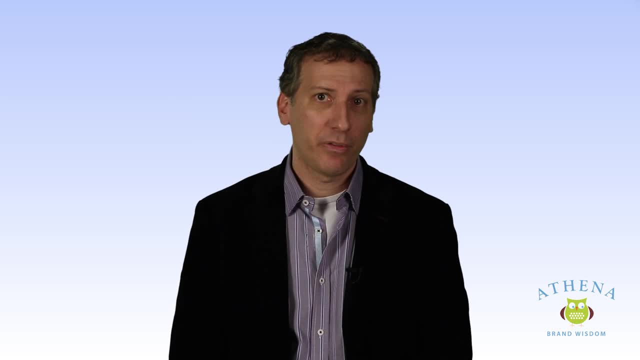 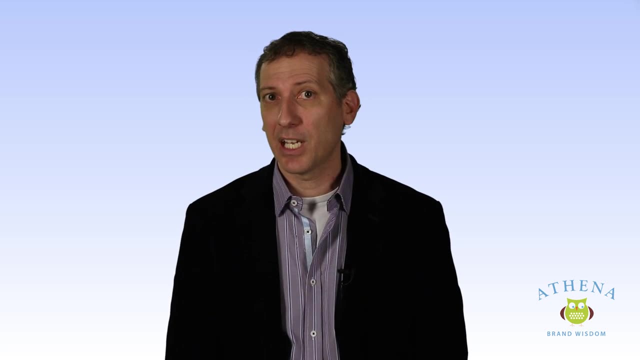 a lot of opinions, but if you give people a pair of scissors, most of them will use it in the same way, And the same is true of websites. So with as few as five user tests or a single day of testing, you can identify the significant usability issues associated. 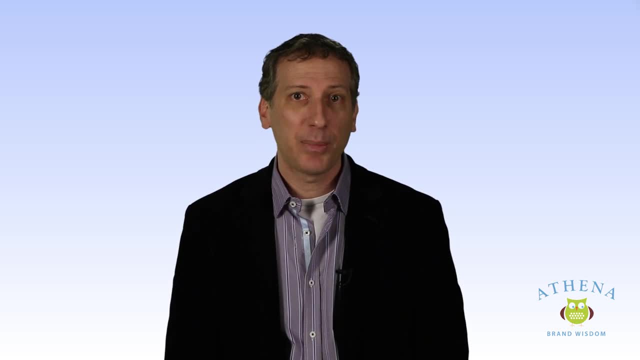 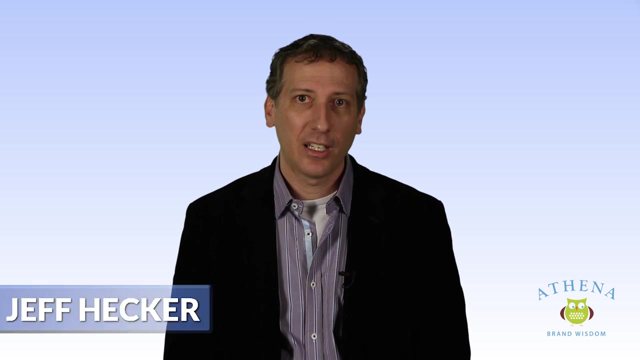 with the set of critical tasks you identify for your site, And that means good usability testing is affordable too. Thanks for watching this video about website usability testing. For a free assessment of how website usability testing could support your site, click the link below and drop us a line at wwwathenabrandcom.